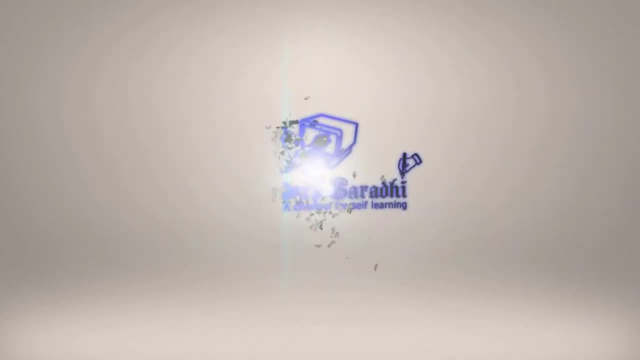 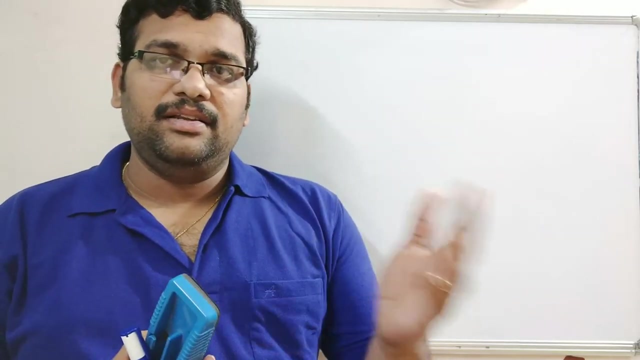 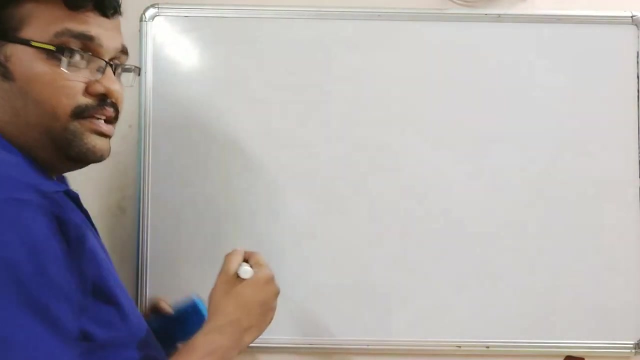 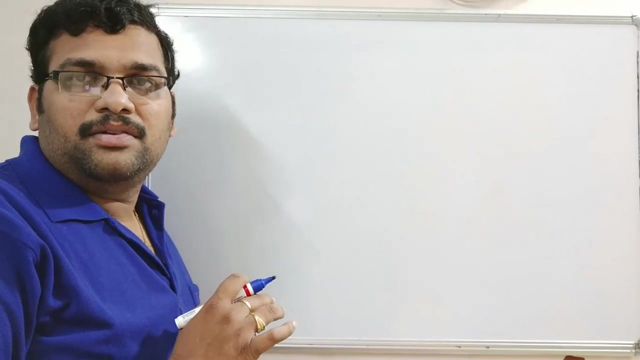 Hello friends, welcome back to our channel. So in this, in the previous session we have seen the structures concept and now we will go with the object oriented concept. So that is introduction to classes and objects. So here the C++ supports the object oriented programming. So object oriented. 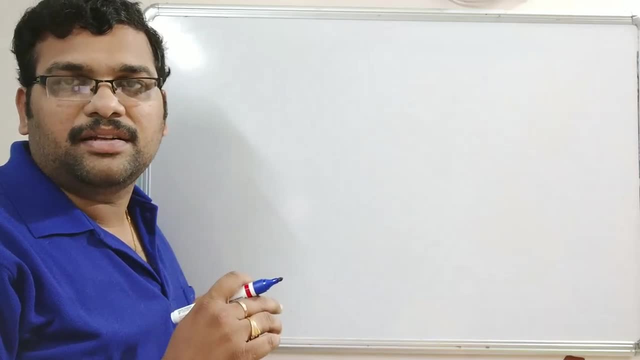 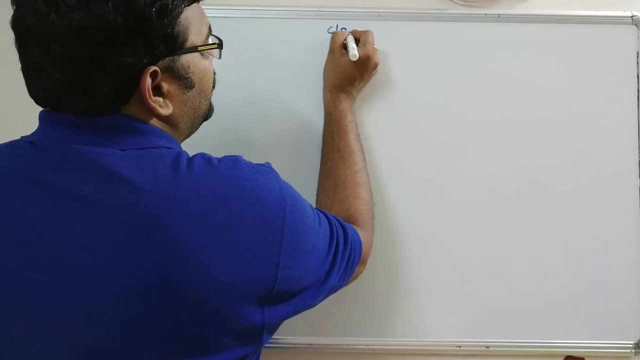 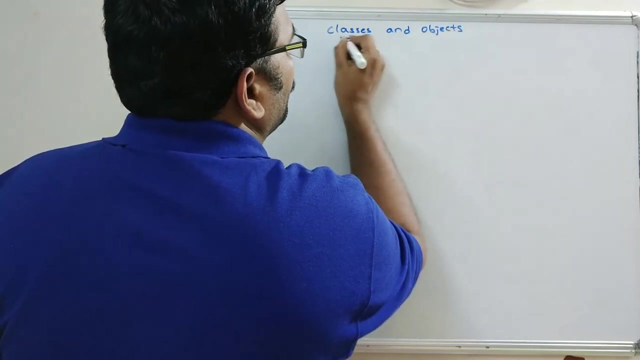 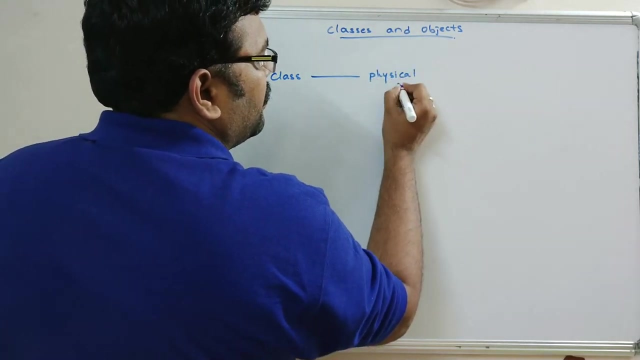 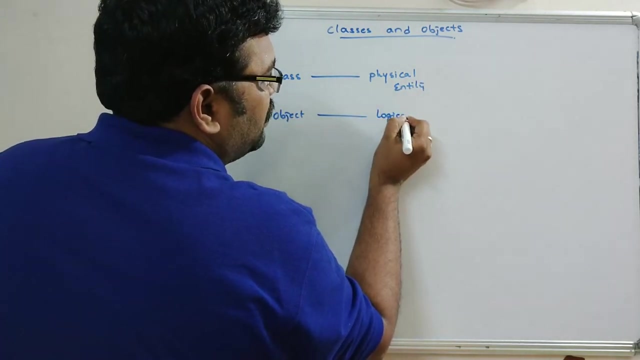 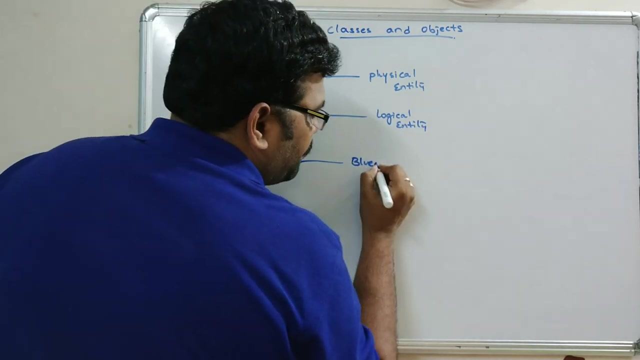 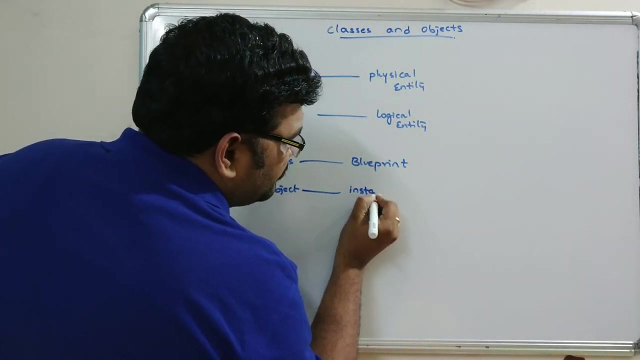 programming means we can write the classes and objects So everything can be implemented with the help of these objects. Now we will see what is a class and objects. So class is a physical entity, Object is a logical entity. A class is a blueprint. Object is an instance of a class. 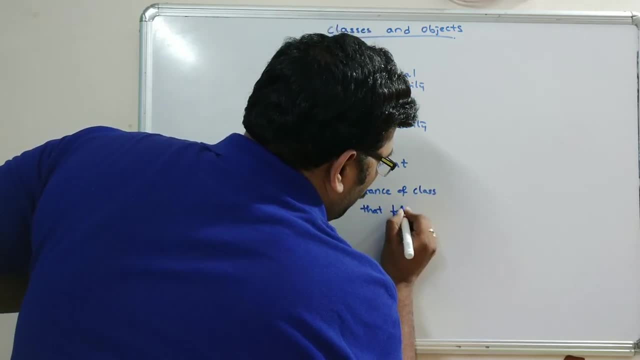 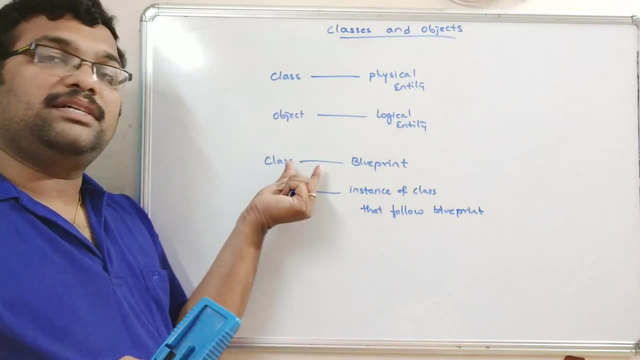 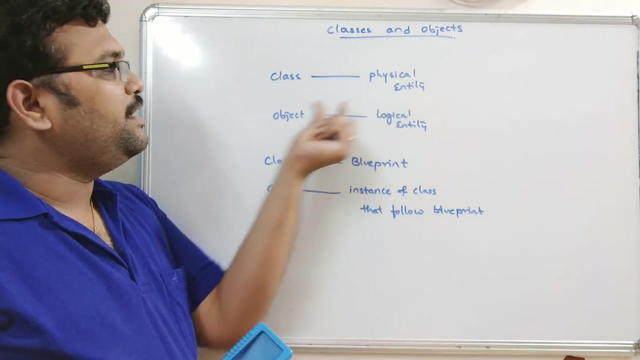 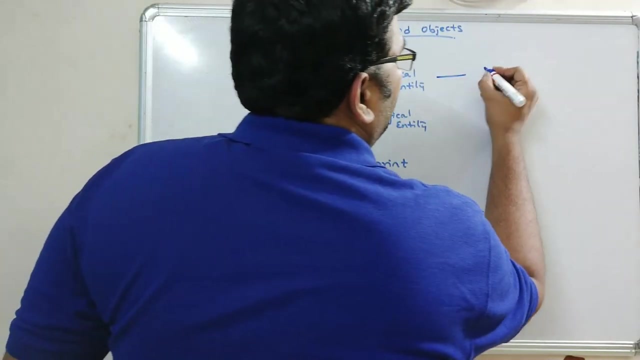 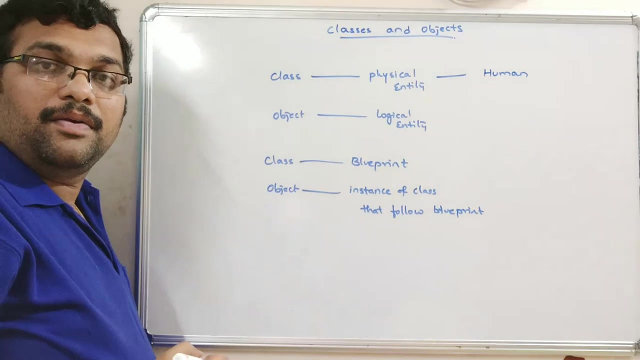 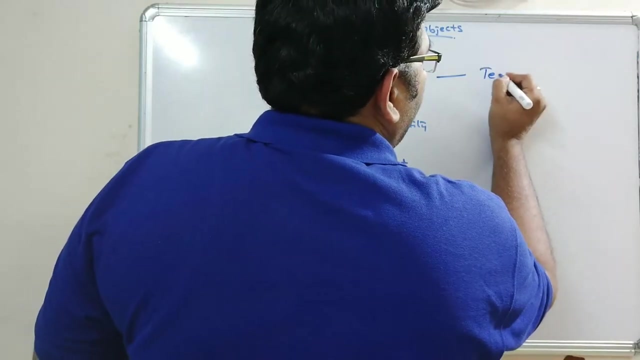 but follow the structure. So class is a physical entity, Object is a logical entity. See, for example, if you write some human, human, or you can go with the teacher, right Teacher. Teacher is a class, Teacher is a class. So 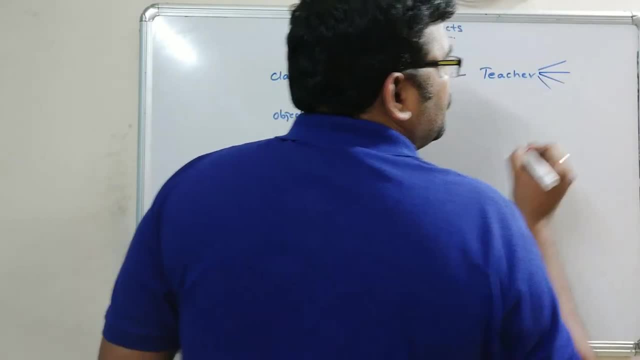 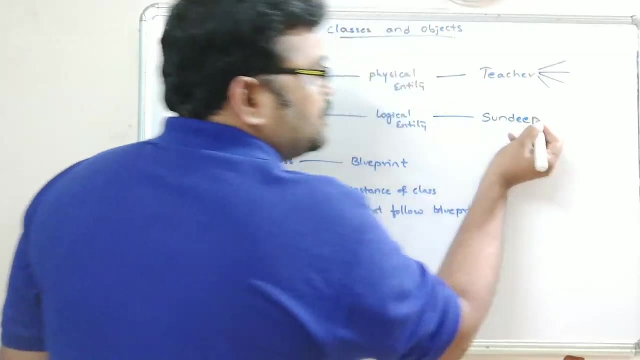 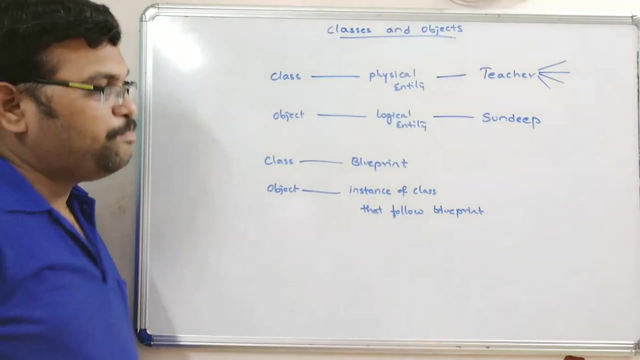 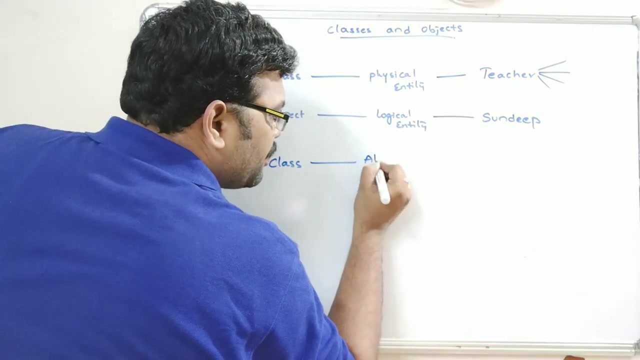 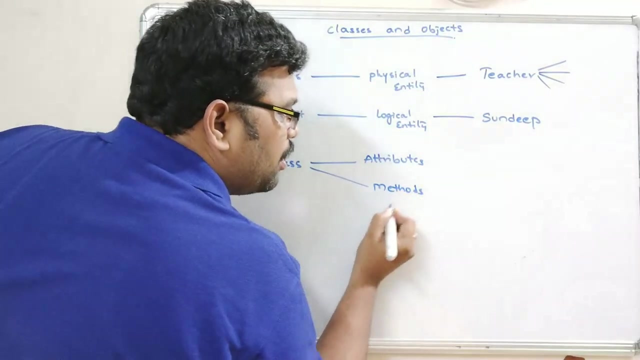 teacher can have the properties, different properties and different methods. right And logical entity is Sandeep. Sandeep is a teacher, Sandeep is an object, So which follows the properties of teacher. Similarly, see A class can have attributes and methods or functions, Methods or functions, So teacher. 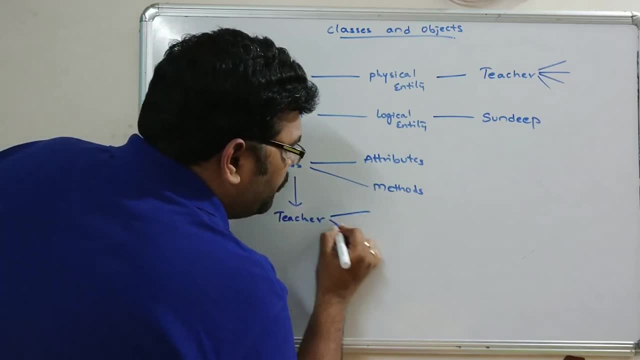 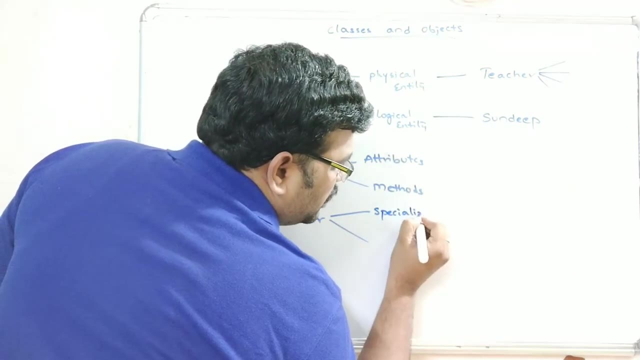 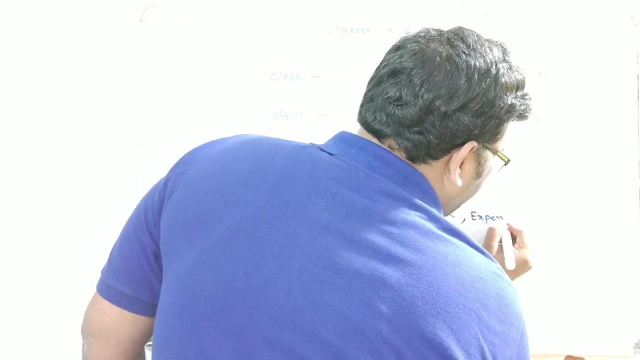 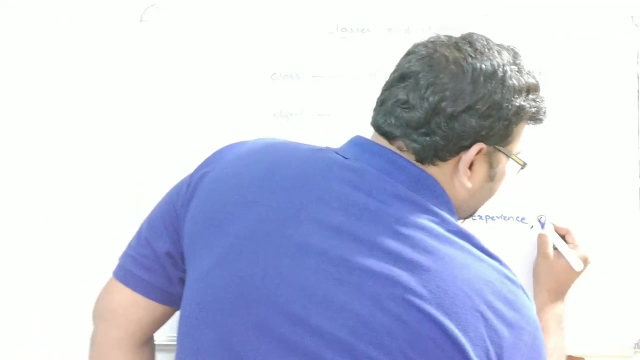 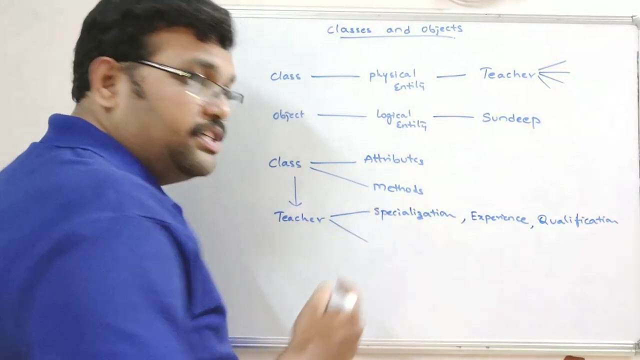 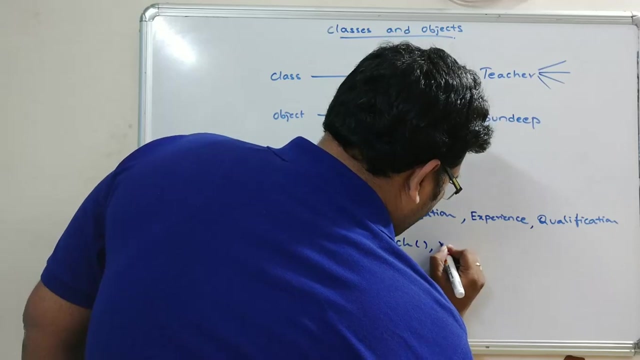 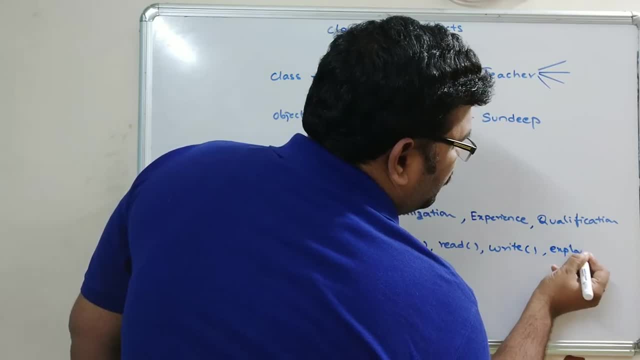 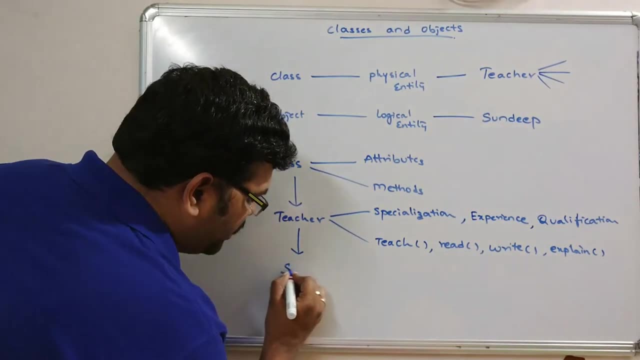 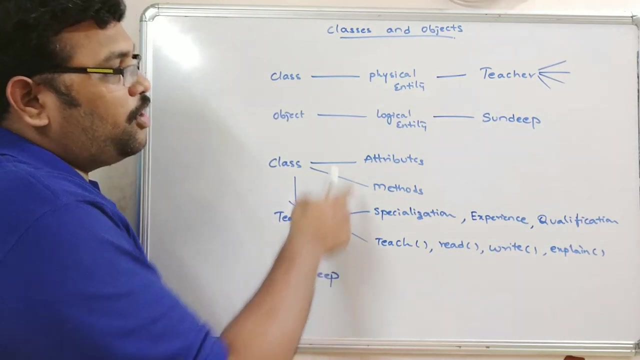 write explain. So there are different functions can be applied for the teacher. Similarly, this is an object. Sandeep is an object of a teacher, class teacher. So Sandeep is an object which is a logical entity which is having a specialization experience. 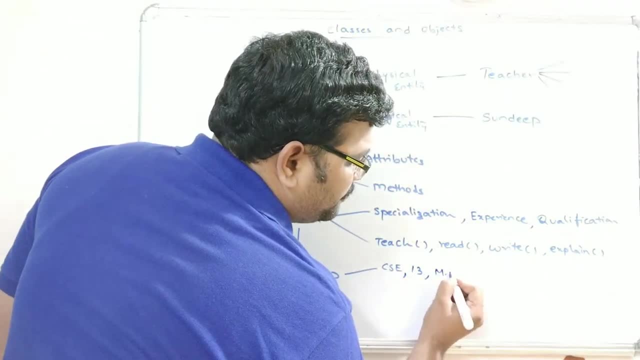 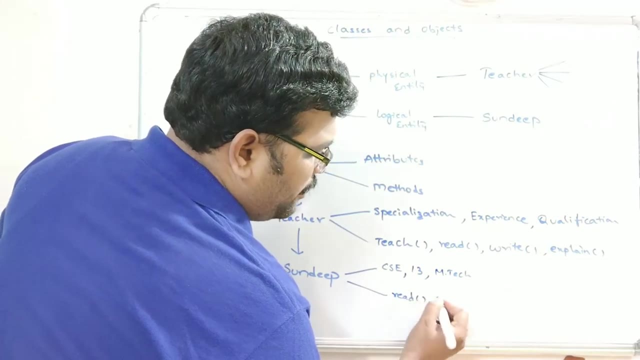 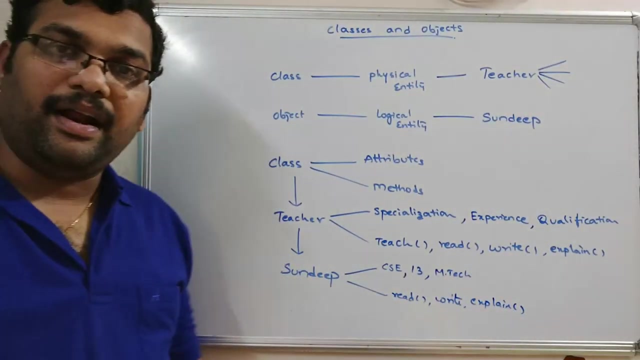 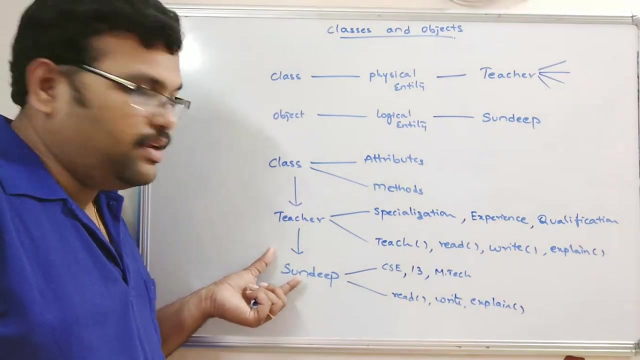 qualification, etc. etc. And coming to this one, so can read, write, explain, Read, write, explain. So Sandeep can read, write, explain. So Sandeep is an object, teacher is a class. 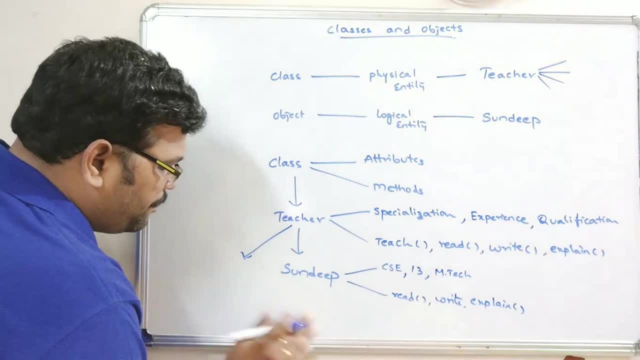 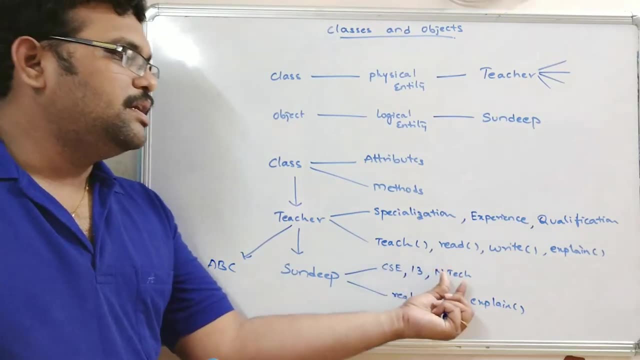 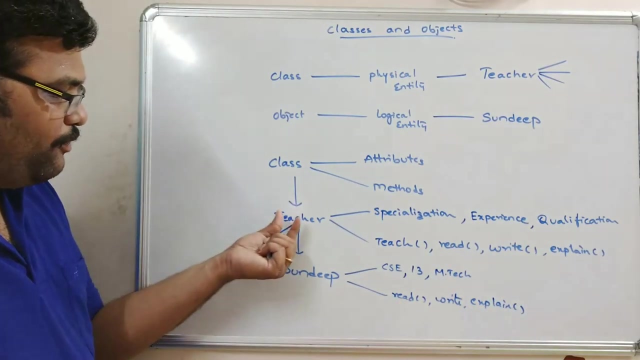 So similar to a Sandeep, there will be some some other teacher called ABC. So ABC will be having some experience, some specialization and some qualification. ABC will be having read, write, explain and so on. So one class. 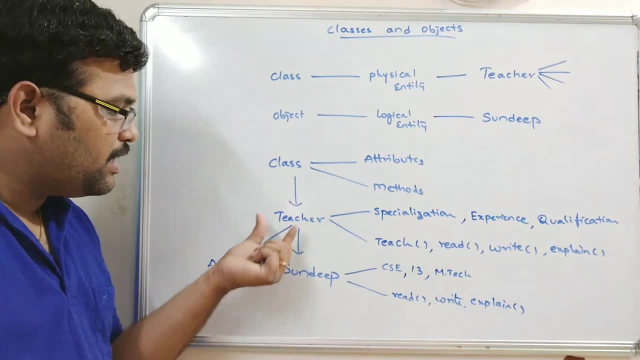 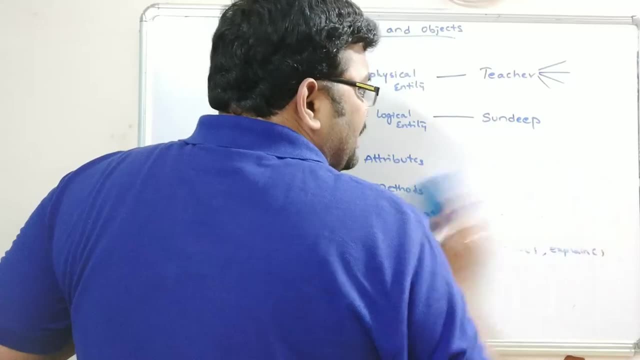 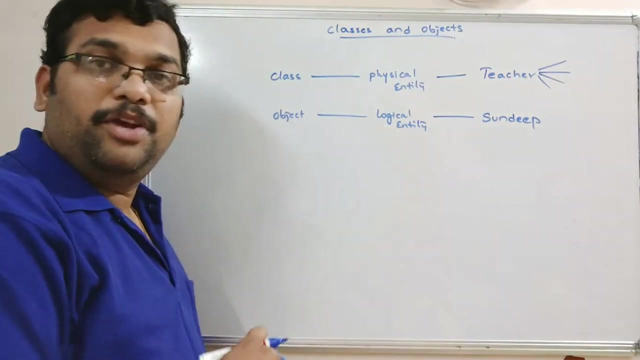 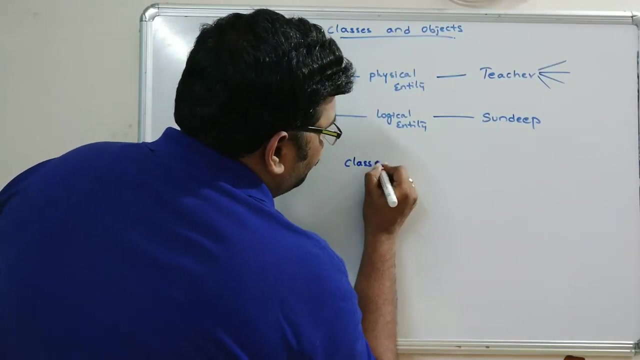 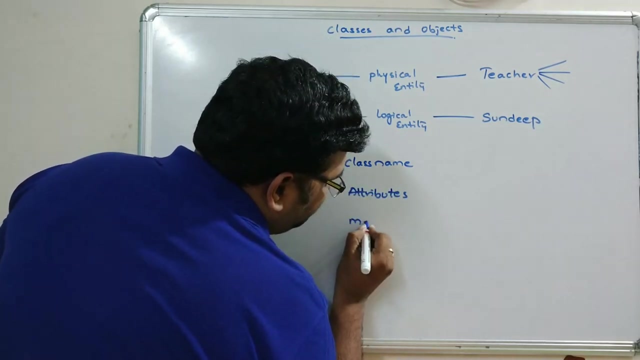 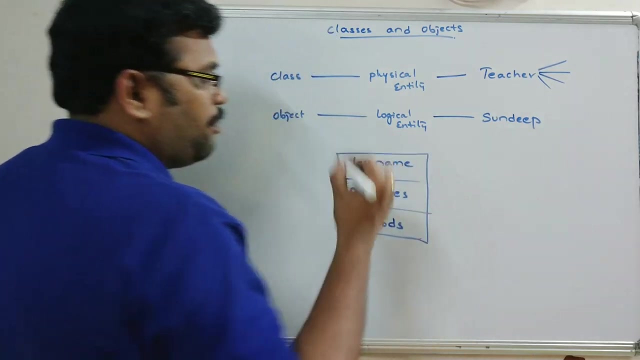 can have a multiple instances. One class can have a multiple objects, Right, See. Just similar to our structure, class will be also having the attributes and methods. So class name, attributes and methods- Right. So we can't access these attributes and methods. 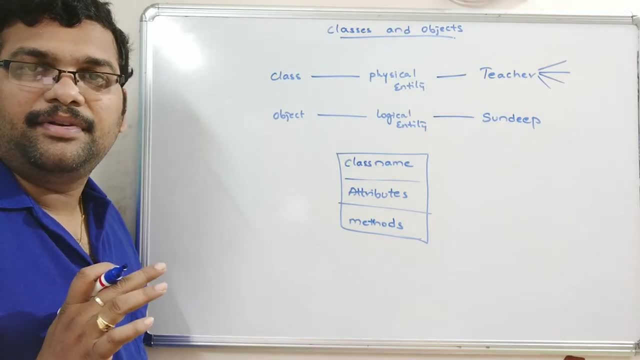 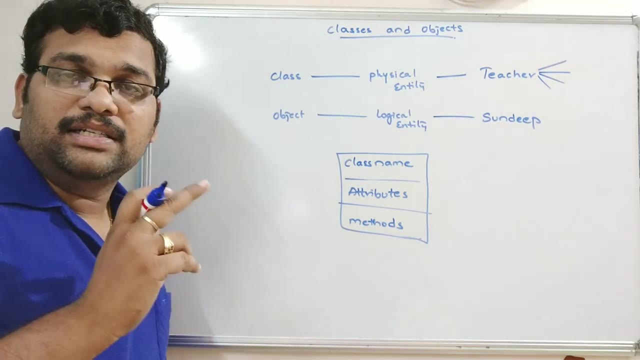 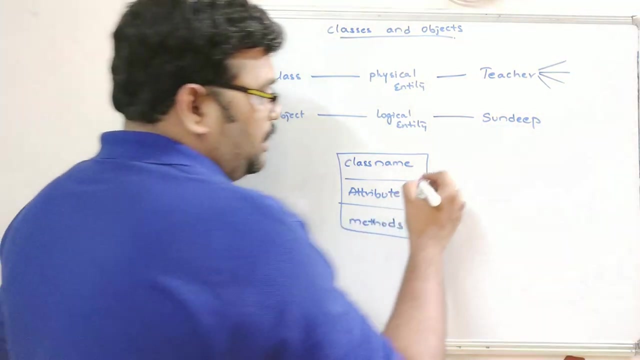 directly, Just like a structure. So how the structure variables can be accessed Through the structure, I mean structure members- can be accessed only through structure variables. Similarly, in order to access these variables and methods, these attributes and methods objects should: 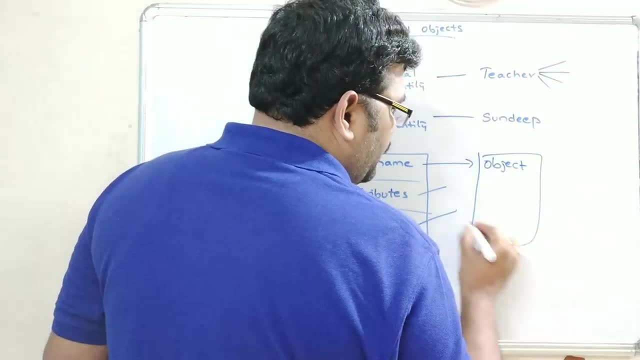 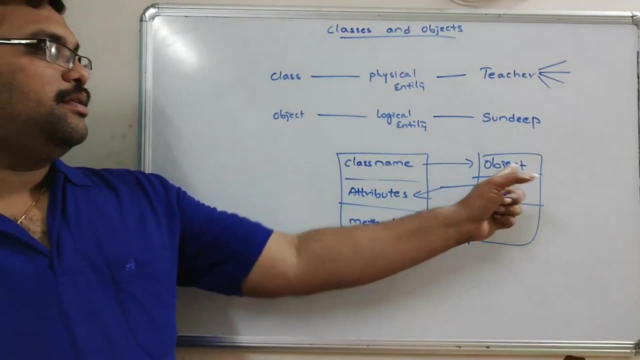 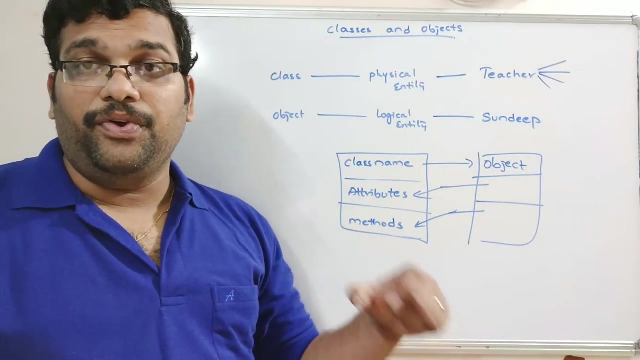 be created. Objects should be created And through the object. the attributes can be accessed. Through the object. the methods can be accessed Only through the object. So if you are creating a class, so we have toIn order to access the attributes or methods. 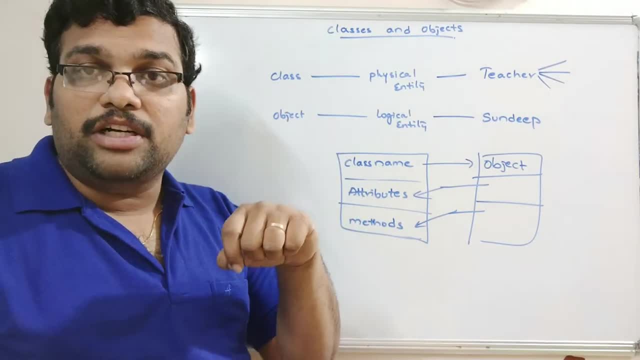 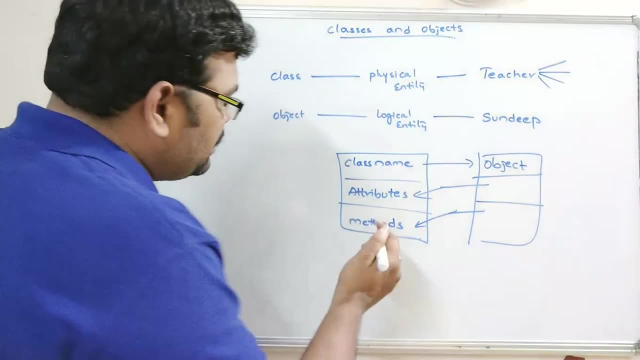 of that class, an object should be created, And through the object only we have to access the attributes and methods. So how to create an object Just similar to our structures? the class name For a bin, For a bin. 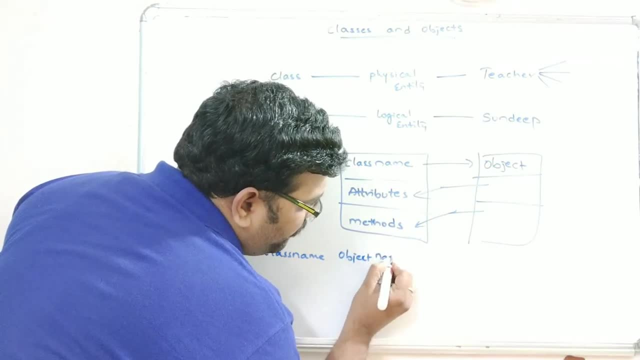 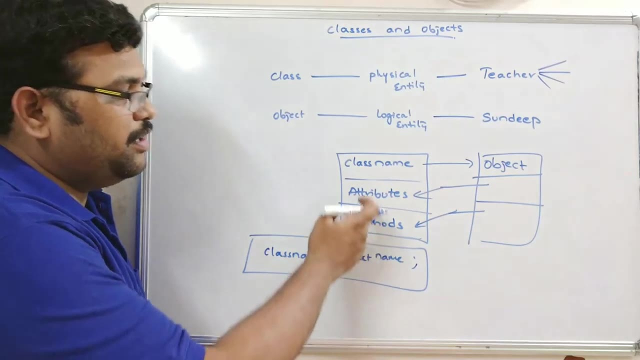 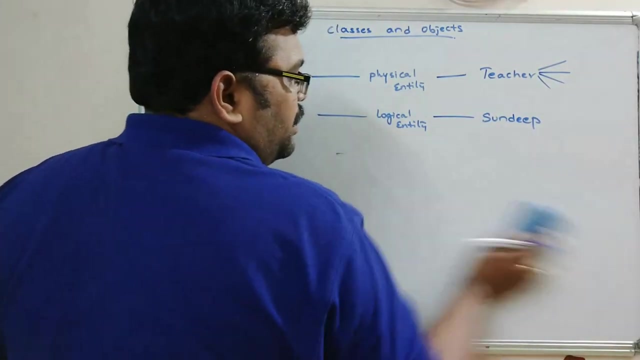 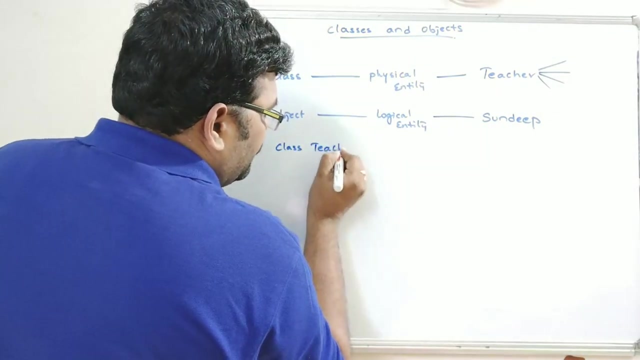 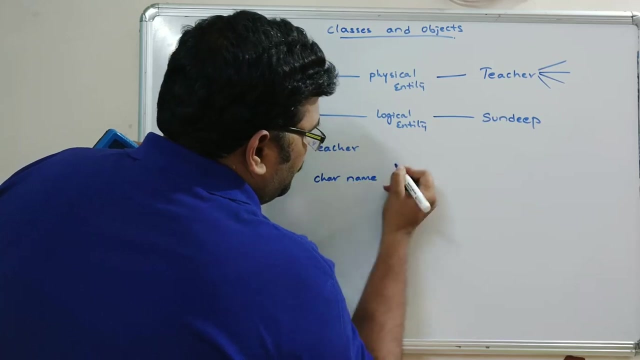 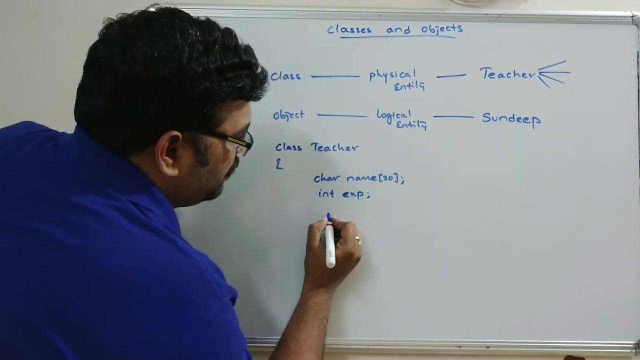 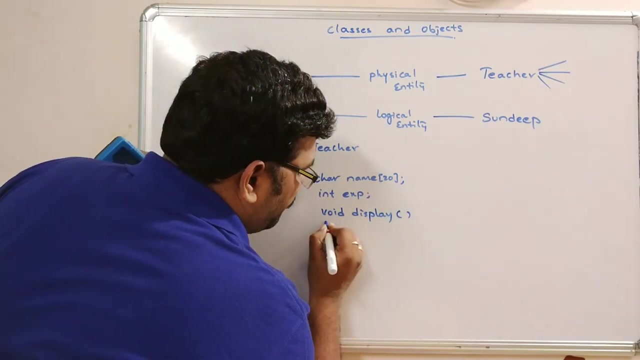 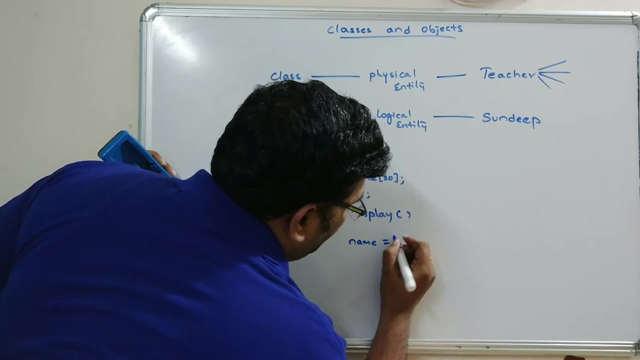 For a bin: object name, class name, followed by object name. object name is created through the object. the attributes and methods can be accessed right. so I will give you a small example and then we'll go with the execution part. so I'm creating a class teacher, so character name int experience void display. here we can write: name is. 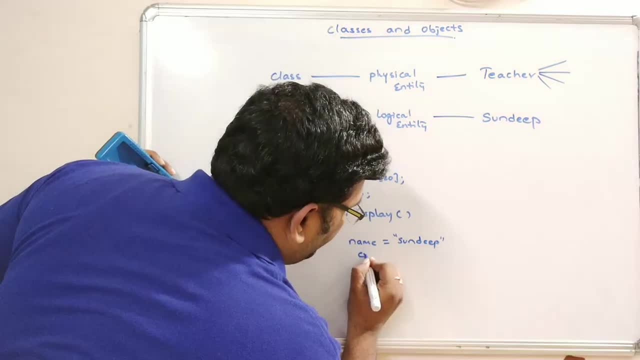 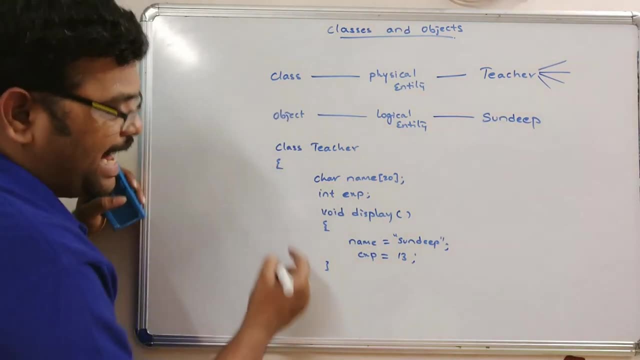 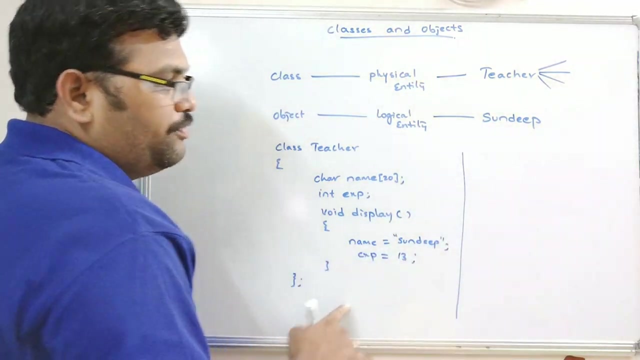 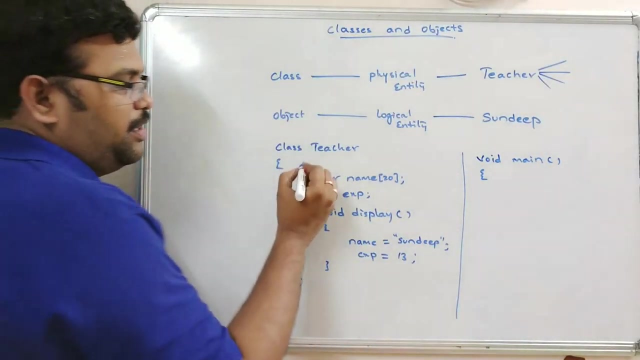 equal to some something. experience is equal to some. 13 and close, and class should be closed with a semicolon, just like a structure. and after comp english of this we have a random, a function for x명이- why me? so here we have to do the scope of these variables as a public, so in the 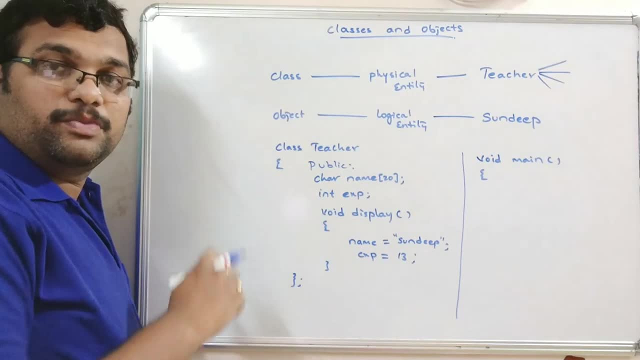 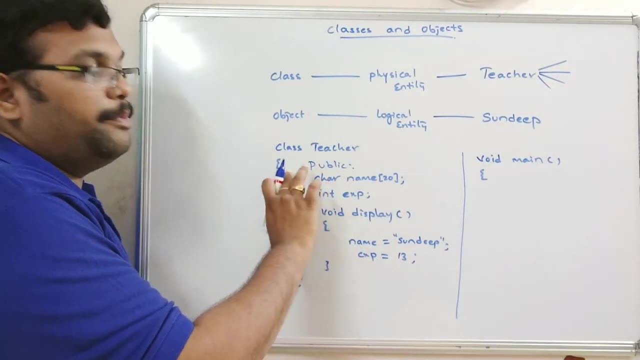 next session I will give you the definition expression of an example. so in the next session I will give you the explanation of the these control space pairs- public, private and protected right. so we will just write down a public so that all the variables and functions will be public. 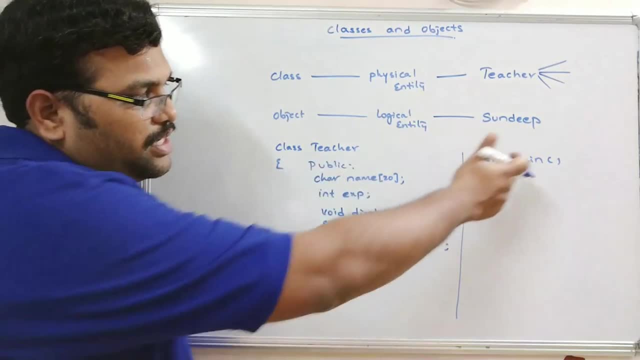 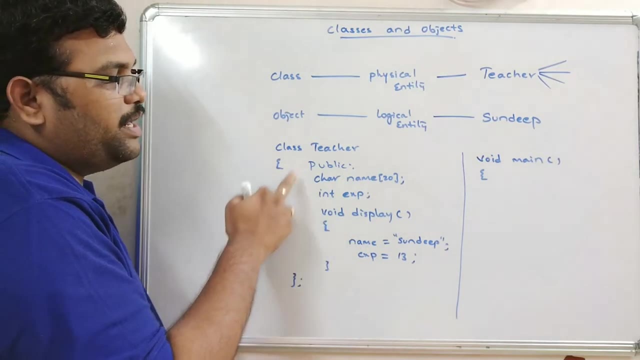 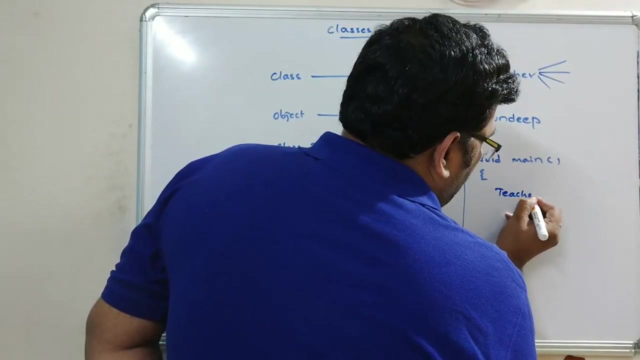 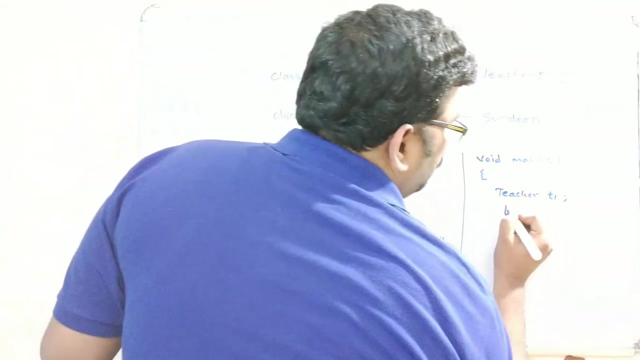 to all the classes, all inside the class and outside the class. so here we have to, in order to access this name and experience and this display function, we have to create an object for this teacher and through that object we can access this one. so teacher t1. so t1 is an object for a teacher class, so t1 dot. 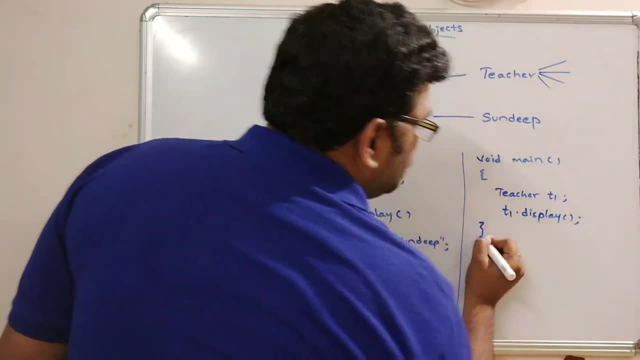 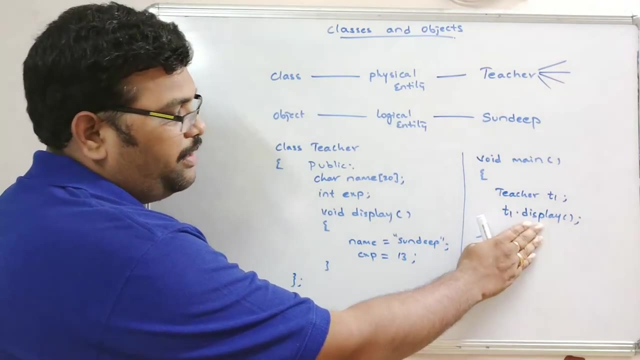 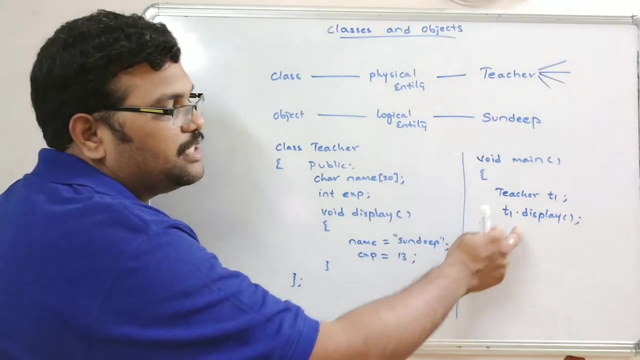 display, automatically this display function will be accessed. so in the absence of this t1 it will not work, because display is a function inside the class. so if the function is inside the class, that that function can be accessed only with the help of object name. so these functions we call it. 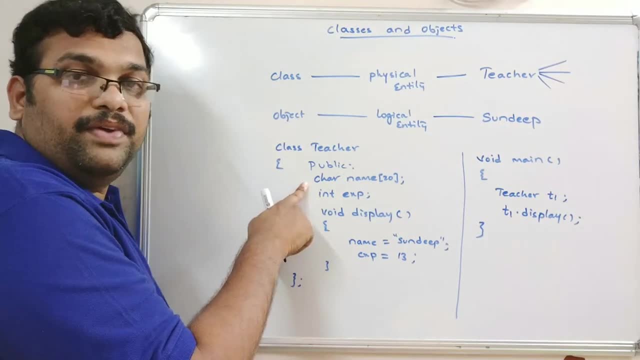 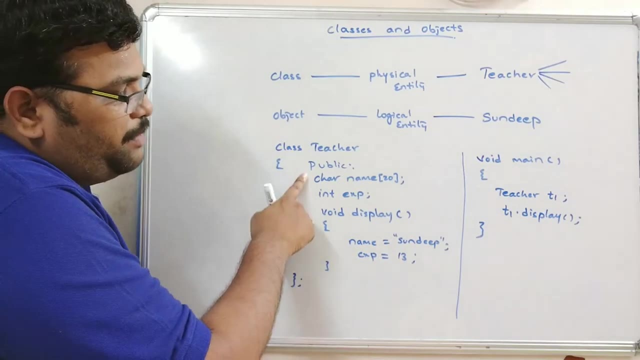 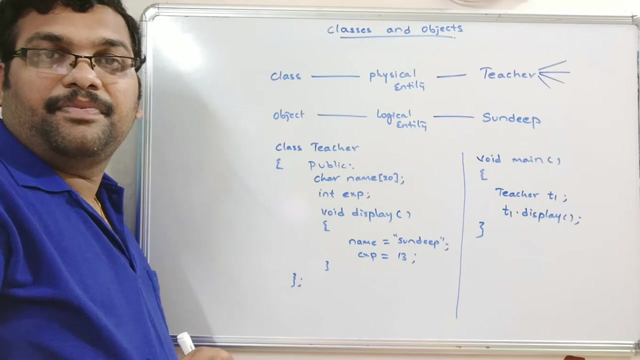 as a member functions. and these are the member variables. okay, class members and member functions, right? in order to access these variables or methods, we have to create an object and through the object only we have to access the variables, right? so hope you understood. these are classes and objects, how to? 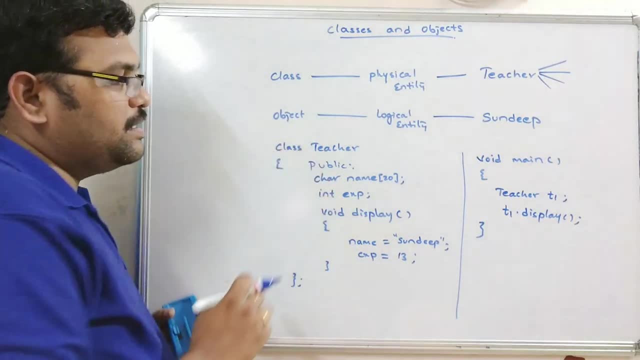 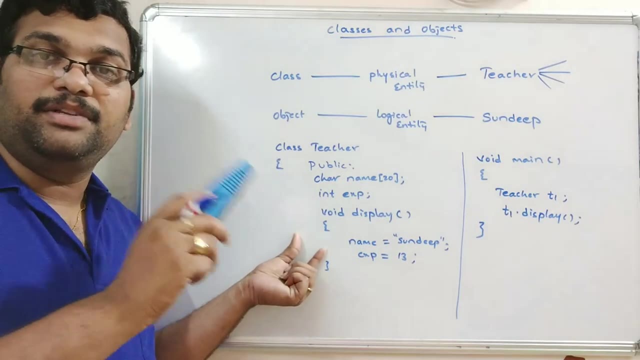 create a class and how to create an object and what are the contents, everything and what are the campus and the material we will be talking about in this video, in the class, right now, till now. so, variables and methods. in order to access the variables and methods, we have to create an object right now. we will see. 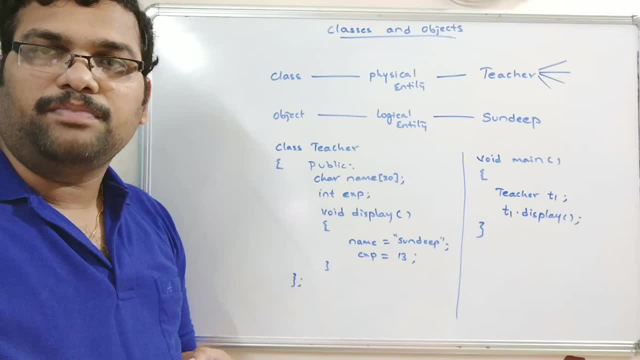 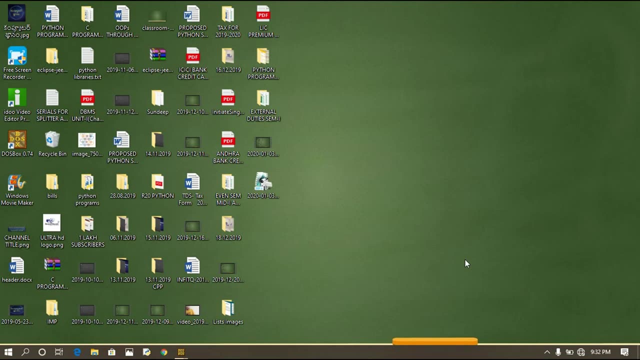 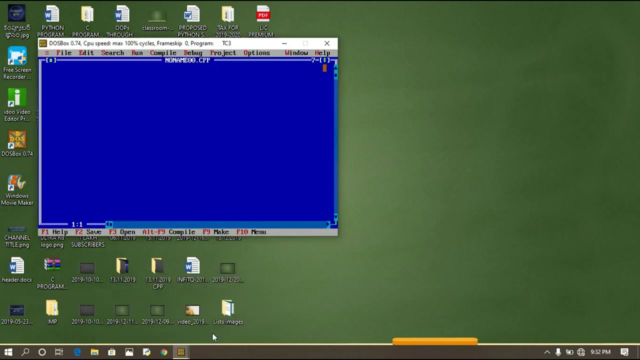 the implementation part of this class and objects. hello friends, so just now we have seen the introduction to classes and objects, so now we will see the implementation of these classes and of the working of this class. so C++ also supports this object-oriented programming, so we can. 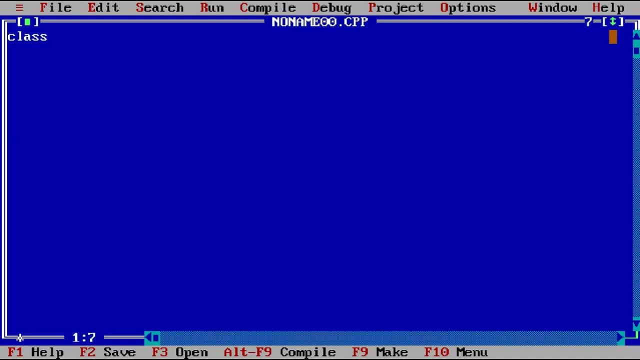 write the class, so we have to give the class name. so let it be. the class name is demo and here you can pass the parameters. or simply we can write the class name as a student and here we can write the attributes or a member, variables and also functions inside the class. so here we can. we have to use the. 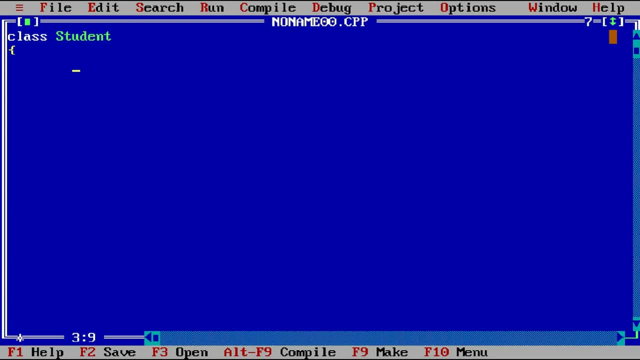 student name and then mention this children name. and here there are three access spacefares. as I have said earlier, there are three access spacefares supported in C++ is public, private and protective. see, if you are not mentioning this public, these access spacefares public, so all the variables will be in a 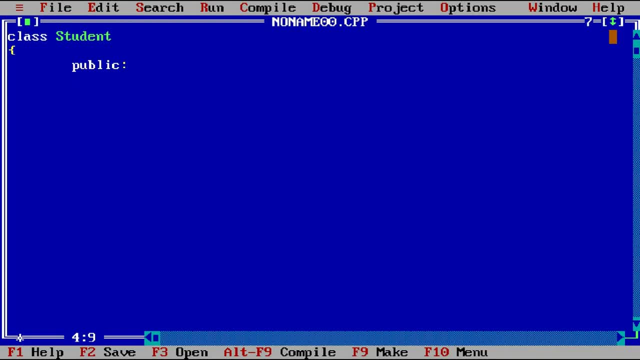 private more so, what's the difference between the public, private and protected, in a public, or declared in private mode or declared in protected mode? So the major difference is scope of the variable, So where we have to use the variables. So if it is a public, 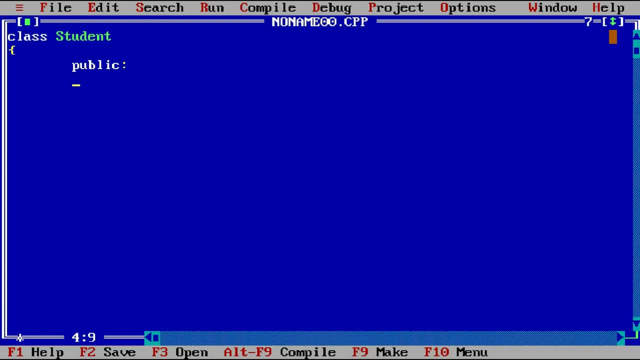 those variables are the functions. So we can use the public in for both the variables and the functions. So if the variables and member functions are public, then those variables and functions can be accessed inside the class as well as the outside the class. Outside the class means 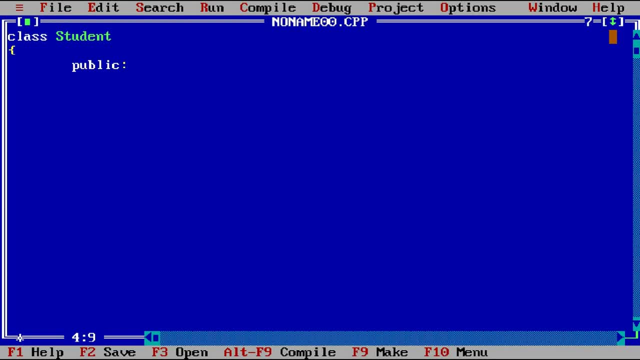 inside the main function also, And if it is declared as a private, then those member functions or those variables can be only used within the class itself. So those variables or functions cannot be used outside the class. Coming to the protected here, it is also similar to our private. 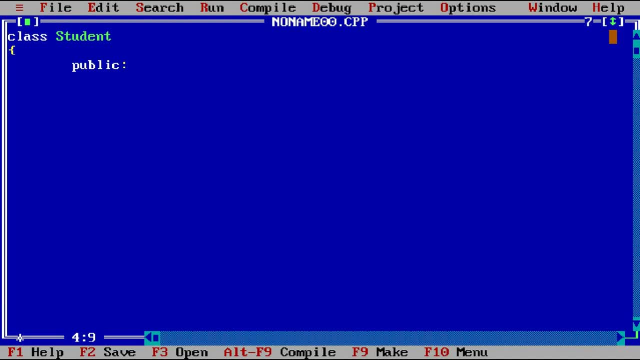 access specifier. But this can be used in inheritance. That means in the inheritance concept. the variables and functions can also be used in derived class, In the base class and derived class. Now let us write the public character: name, int, r, number. Right Now I will write the main function. Also, we can write the function here. We will write the. 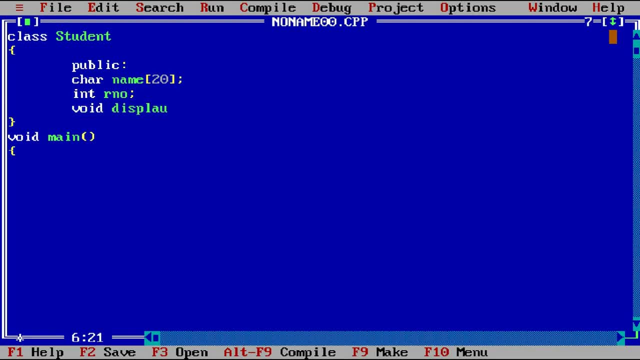 function also void display Similar to over structure Inside the class. Right Coming to the main function here. So if you want to access the name, roll number and the display, we have to create an object for the student and through that object we have to access. 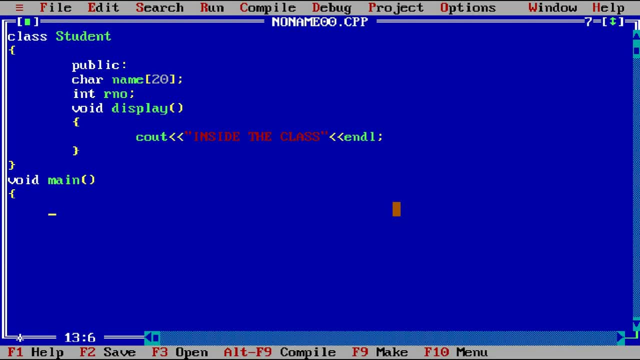 the name and roll number, Just what happened in this structures concept, The structures concept, The structure. also. In order to access the members of a structure, we have to create the variable structure variable and then, through the structure variable only, we have to access the methods. I mean. 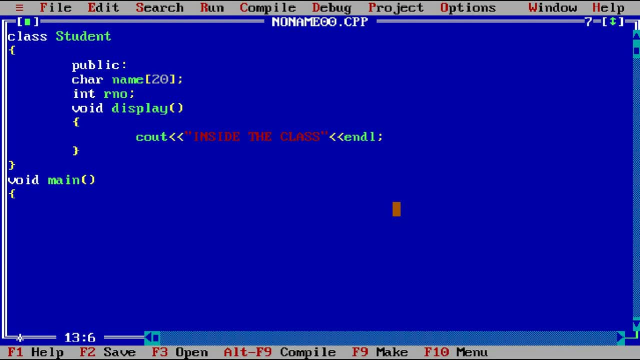 functions or the variables. So here also same, But here we are declaring it as a class. So here we can use the control specifiers so that data can be hidden. So here I am creating this Object for the class With the help of this one. So See out, Enter name. See in: Yes, dot name. 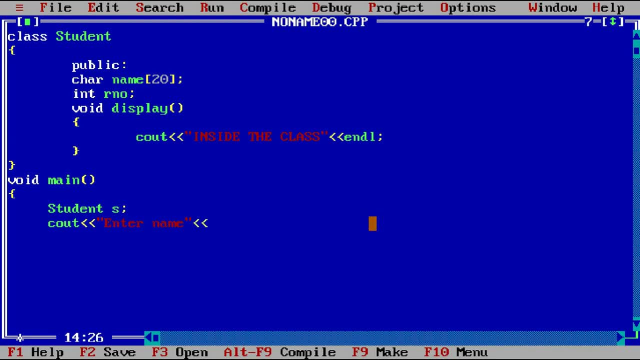 Object for the class. With the help of this one. So See out Enter name: See in Yes dot. name. Object for the class. With the help of this one. So here we have created the variable And then Simply you can write Yes dot Display And See out Enter name: See in Yes dot. 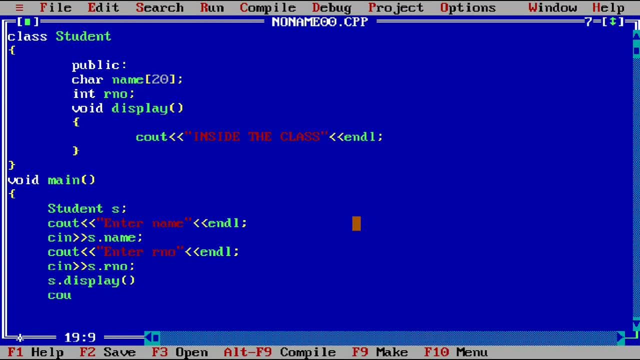 R number And then Simply you can write Yes dot Display And See out Enter name. See in Yes dot a stock name, R number right. So let us save this one, classcpp, save this. so we are having yes, there are no header. 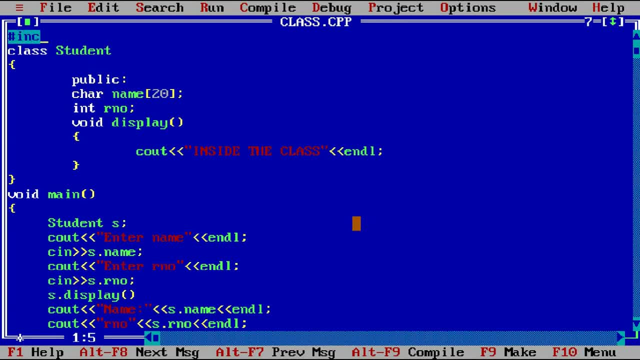 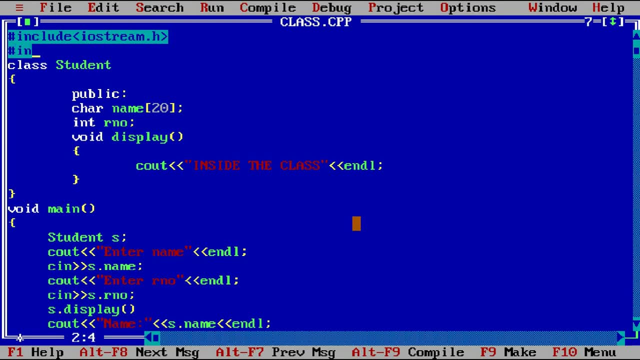 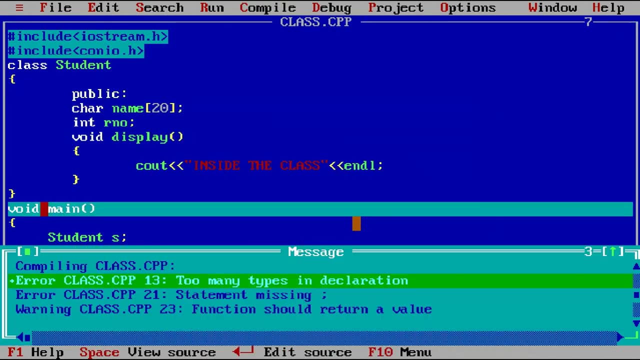 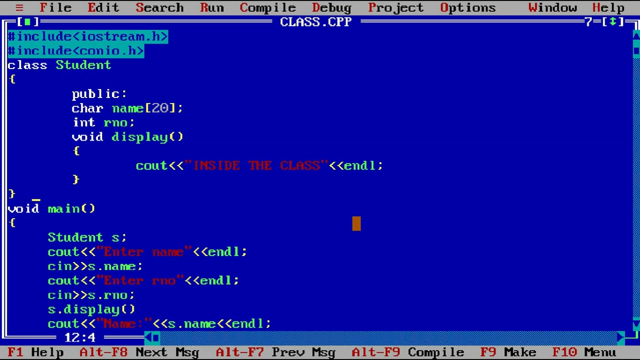 files. we have not included any header file here. So hash include iostreamh, hash include conjoh and then hash include iostreamh. two more two minute types declaration. so here we have to keep the semicolon. that ends. 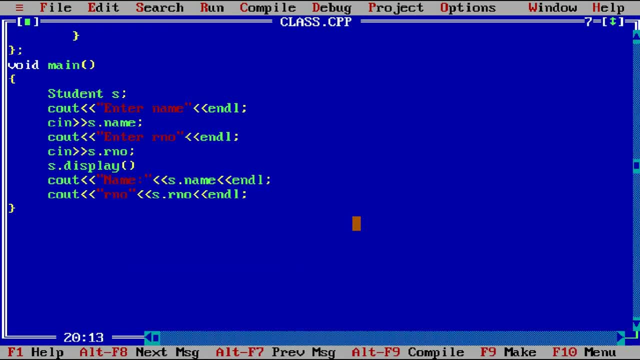 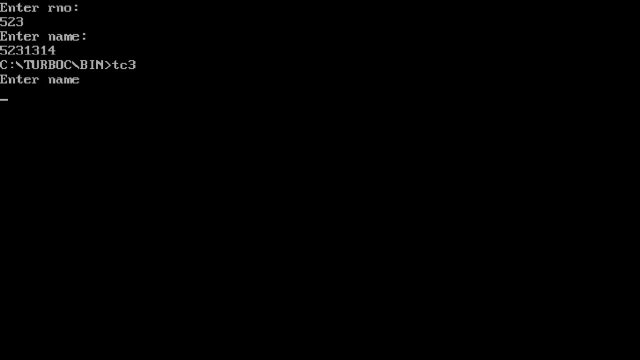 the class. so statement missing the semicolon here. once again we have missed the semicolon. right Now let us execute this one. so enter name: so again I am giving Sandeep. enter R number: again I am giving 523.. 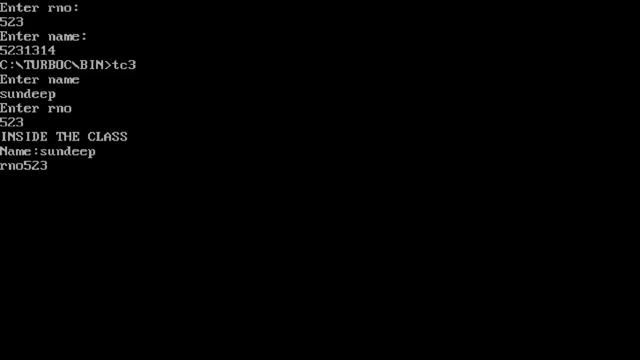 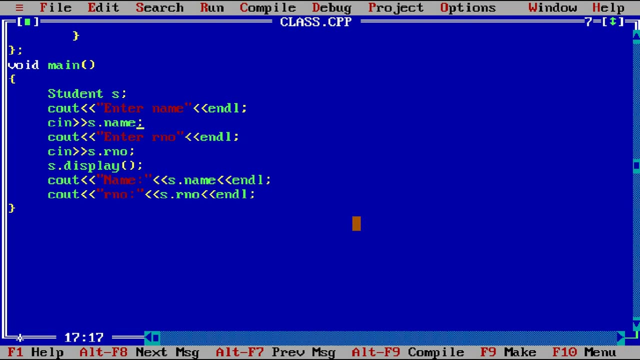 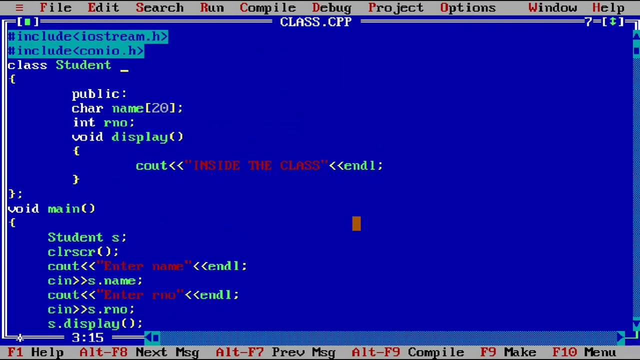 Now you can observe The result inside the class name: Sandeep R, number 523,. yes, so, similar to our structure, a class can be implemented. the difference is here. we can use the access specifiers. 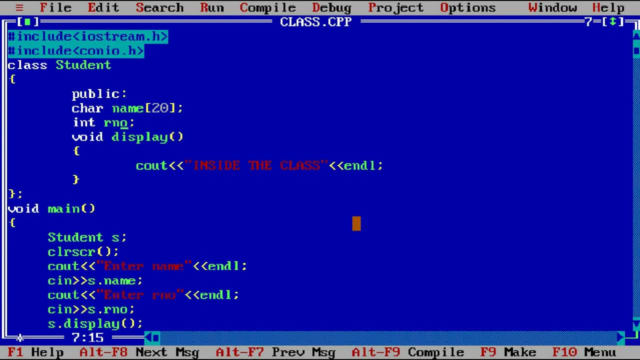 the control specifiers is a public, private or product. If you are not giving any Anything here, by default it will be as a private. see, as this is the public, so these variables and the methods can be accessed outside the main, outside the class also. 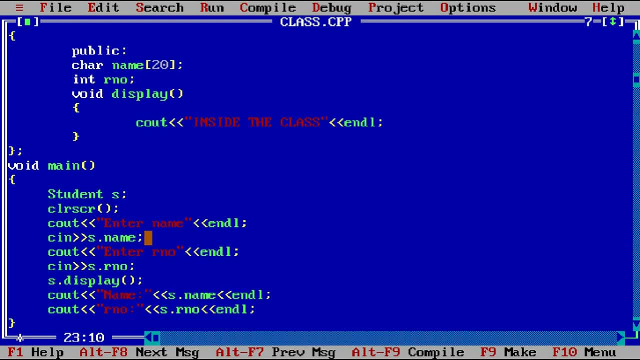 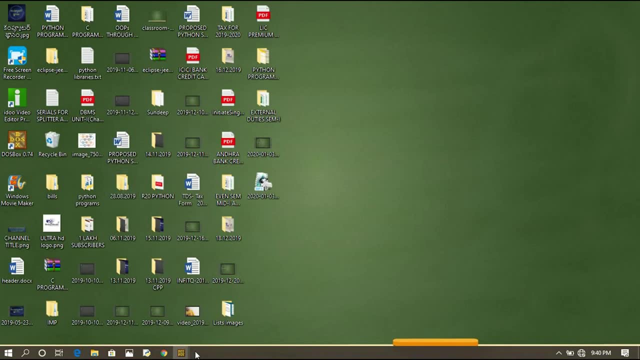 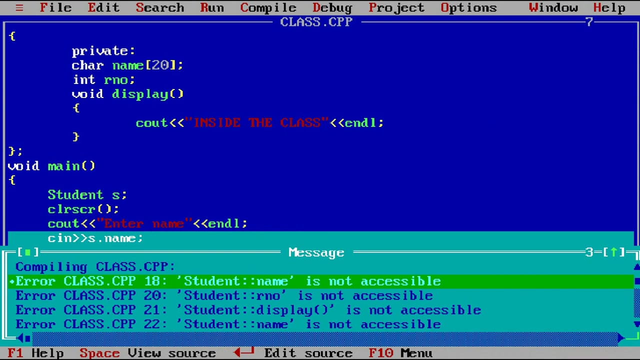 so in the outside the class, that means inside the main function, we are accessing the methods in the way this one. see, if you created here private, we cannot access. sorry, private private. Okay, So if you compile you will get an error. student name is not accessible. R number is: 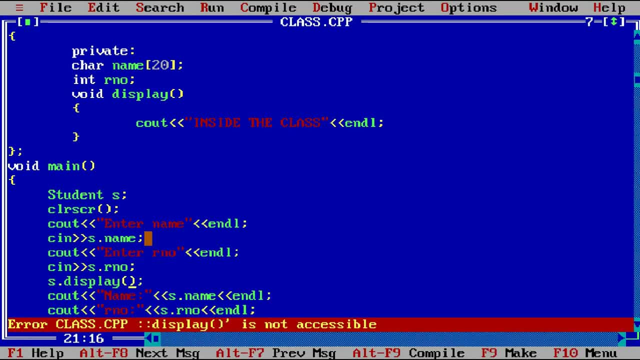 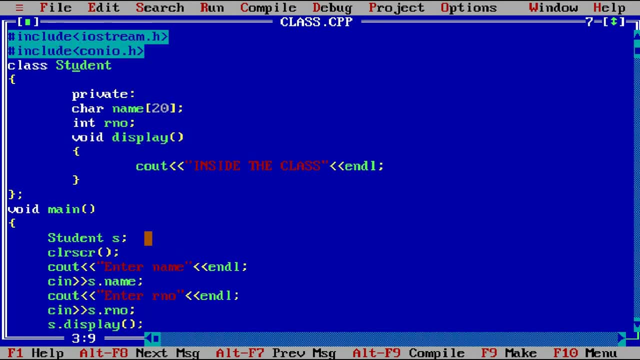 not accessible. display is not accessible because these variables and functions are declared in a private scope. that means data is hidden, so these can be accessed only inside the class itself. Okay, So here you can write here. see out, enter the name. 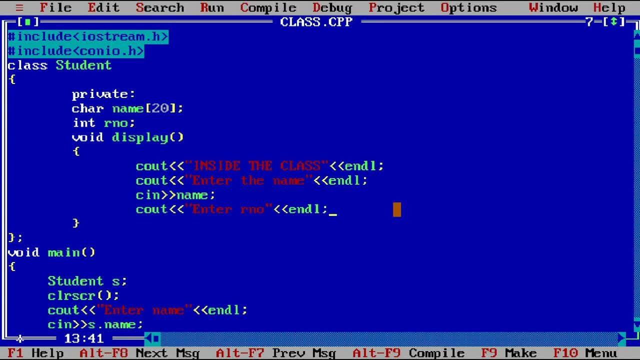 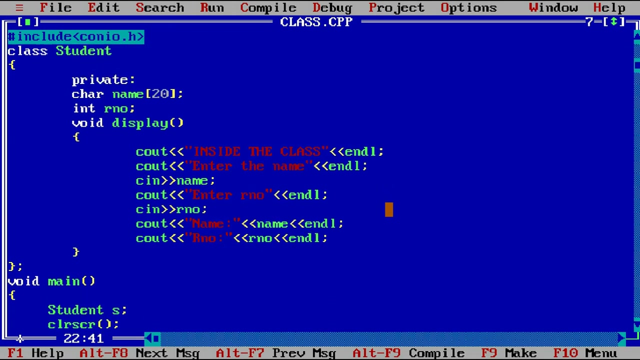 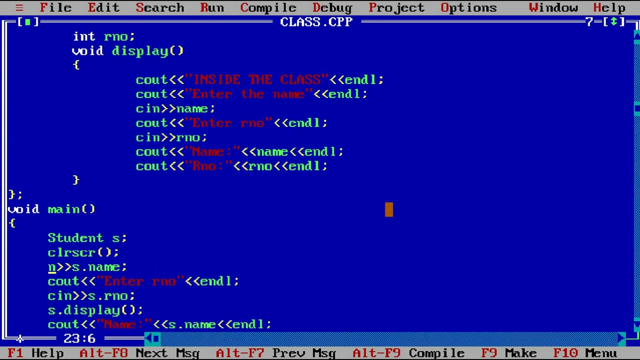 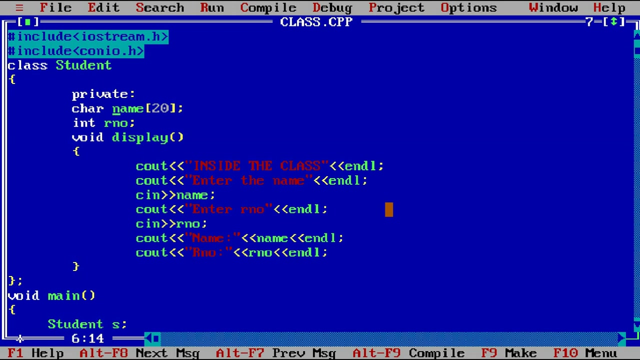 Right, See, now here I am completely removing all these things and just I am calling this function. and again here I am removing all these things And see, this name is private, R number is private, So these can be accessed only inside the class itself. 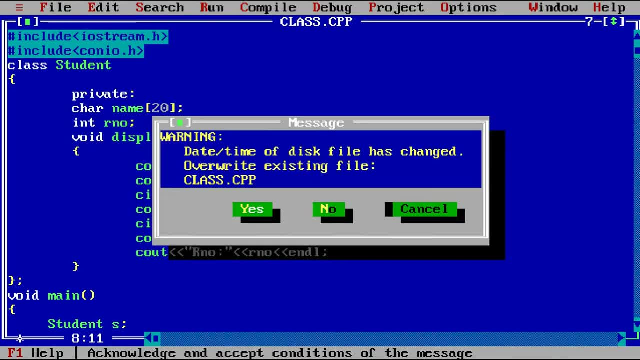 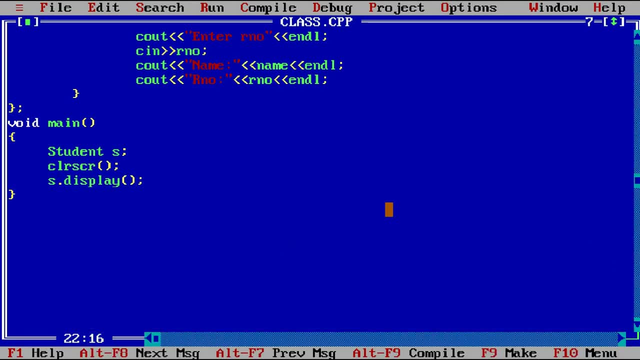 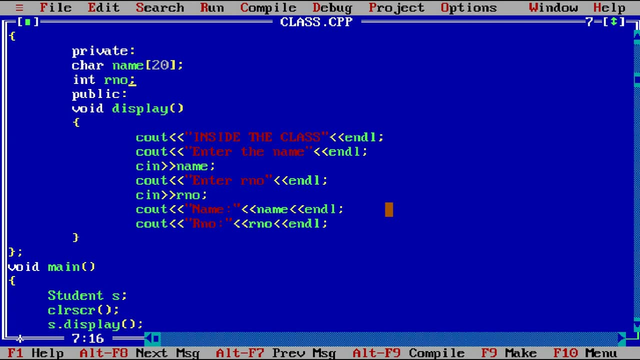 Also, this display is also inside the private. So again we will get the error because we are using this display inside the main function. that means outside the class which is declared as a private. So if you change the scope of this method as a public, see private. 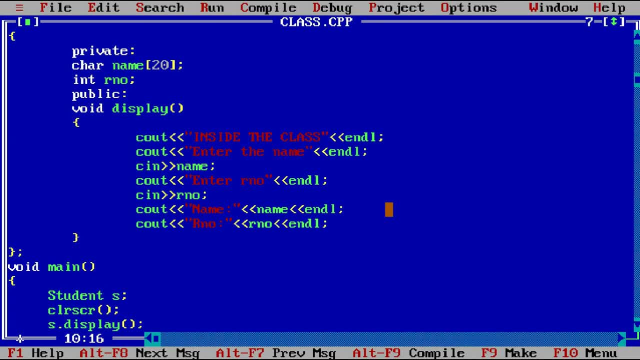 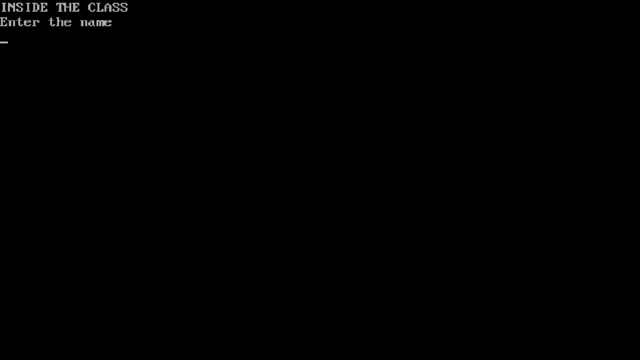 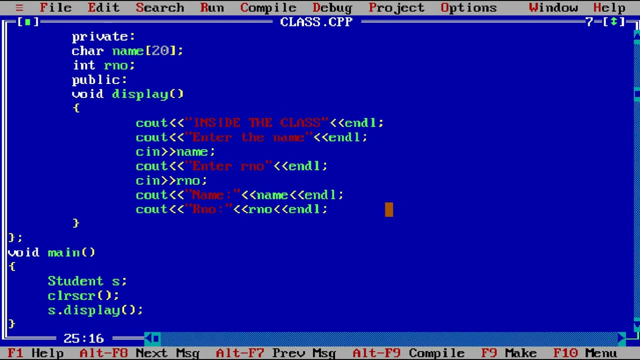 These two variables are in the private And public. the method is in public. Now the display function will be worked. See, you can observe here: enter the name Sandeep 523.. And you can observe here: see name is Sandeep R, number 523.. 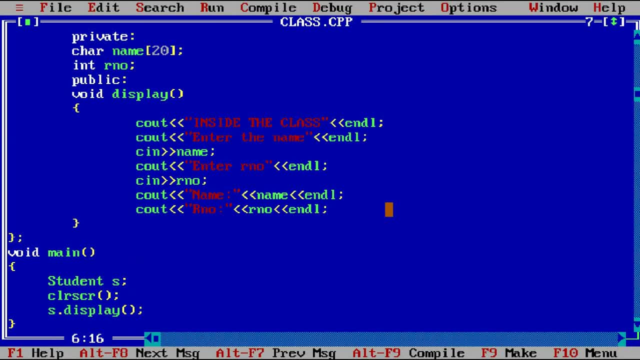 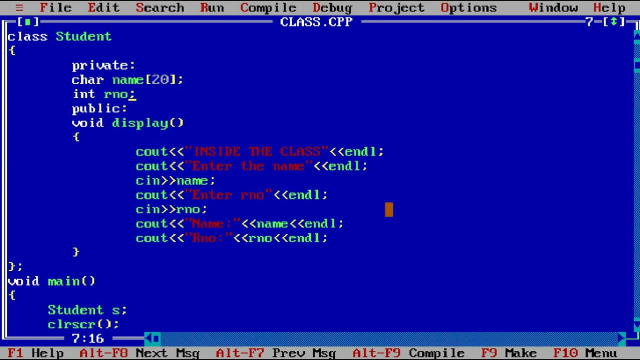 Because these name and R numbers are private, so are in a private scope. that means these variables can be accessed only inside the class, So they cannot be used outside the class. So in main function we can't access this name and R number. 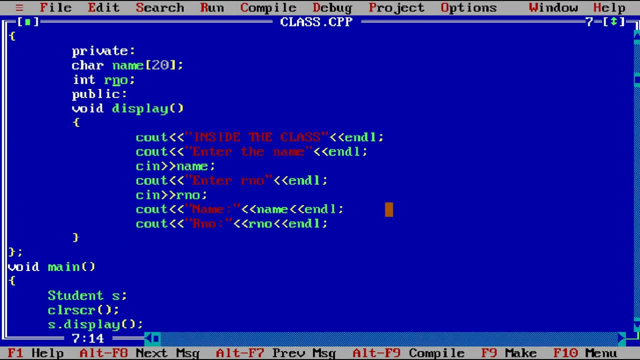 Even though we are creating the object for the class, we can't access this name and R number because the scope of these variables will be in private. And coming to this display function, we have changed this scope as a public, So display function is a public. 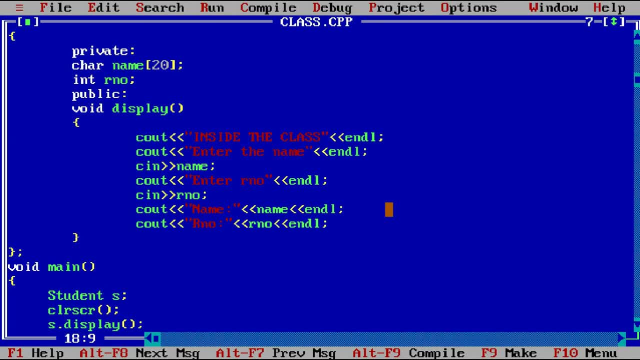 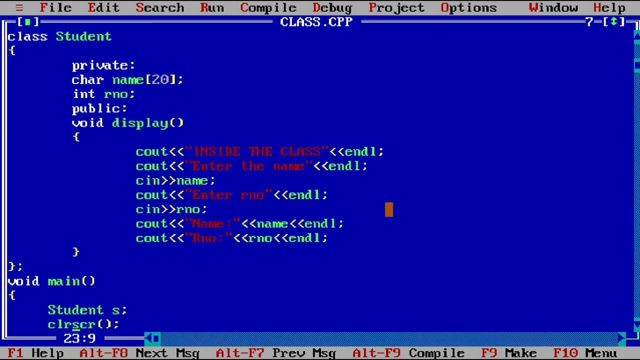 So this function can be used inside the class as well as outside the class. So outside the class means inside, outside the class, with the help of the object created for this particular function. So in the main function I have created an object for the class s and I am calling this function with the help of object sdisplay.